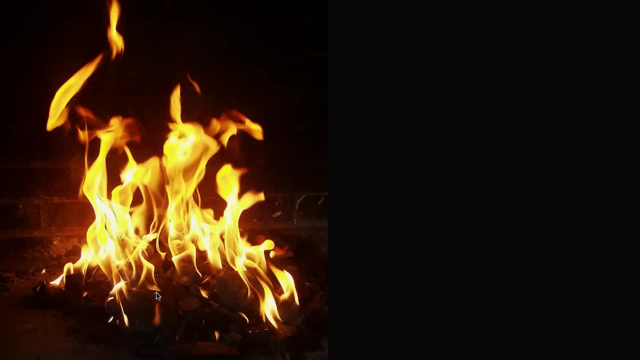 When we observe what we call fire, we have this combustion reaction going on and then we see these flames. what we're really observing are the three forms of thermal energy transfer. We're observing conduction, conduction, convection, convection. 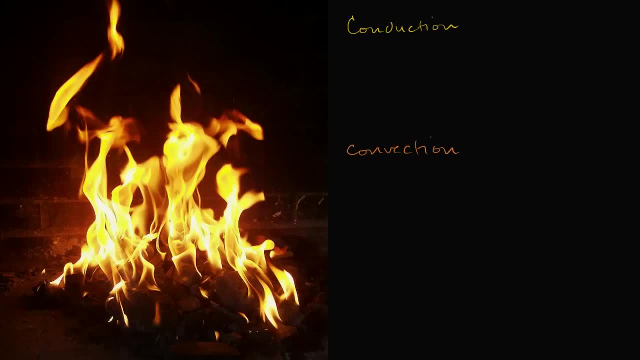 convection and thermal radiation all at the same time. So it is thermal, thermal radiation, thermal radiation, And I could say thermal conduction, thermal convection and thermal radiation. The word thermal is just relating to things dealing with temperature. 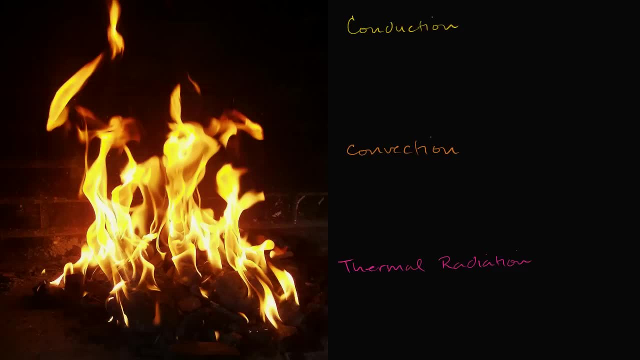 So what is the conduction going on? Well, what we have going on in the fuel for our fire. so down here, the fuel for our fire, we have our classic combustion reaction, and I encourage you to watch the video on that in our chemistry playlist. 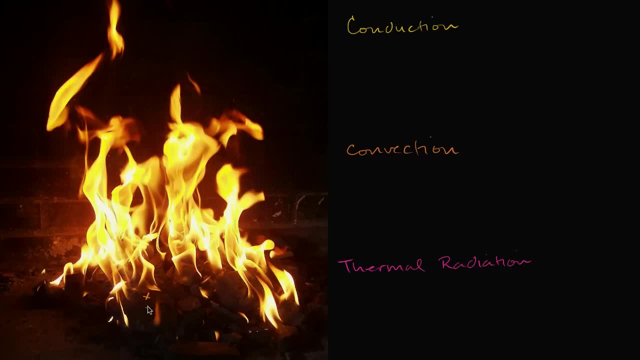 Or our chemistry section if you're interested in it. But you're taking carbon molecules and their bonds and then, in the presence of oxygen and some heat, you have a combustion reaction producing carbon dioxide and producing water and even more energy than you put into it. so it's producing a lot of energy. 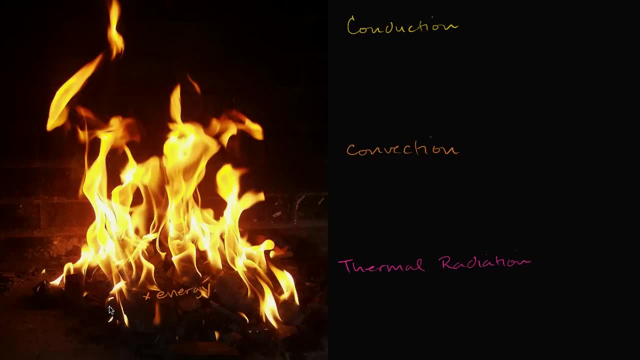 And that energy is going to excite the molecules that are around it. so you have these molecules. you have these molecules that end up getting a lot of kinetic energy- and remember temperature is proportional to average kinetic energy- And so the ones that just combusted 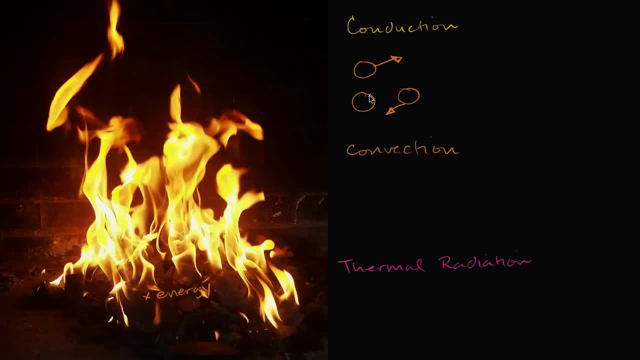 or the molecules right near the reaction, or maybe the ones that were part of the reaction. they're gonna have this really high. they're going to have this really high average kinetic energy, Because all of this energy was released from that combustion reaction. 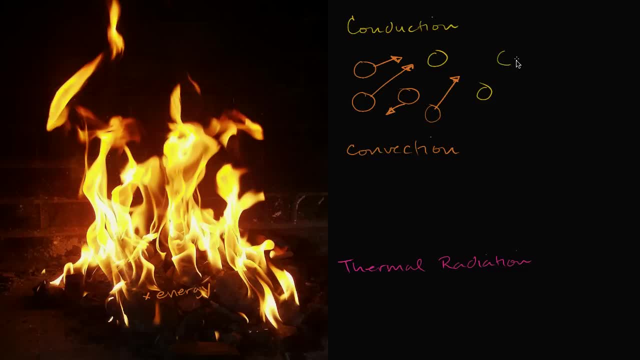 And then they're going to bump into other molecules that might not have quite as high kinetic energy, but then they're going to transfer that kinetic energy through these collisions And I could have a whole video on thermal conduction. but that's what's happening. things with higher 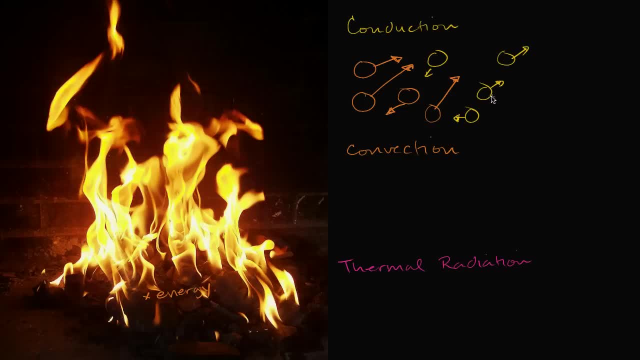 kinetic energy are bumping into things with lower kinetic energy and transferring some of that kinetic energy and they're transferring some of that momentum. So that is definitely happening when we look at a fire like this: that neighboring molecules are bumping into other molecules and transferring energy. 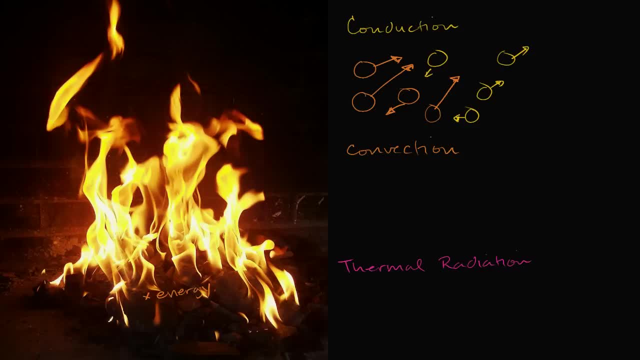 Now convection. this is around the idea that hot air is less dense. So if we have a bunch of air particles here, so let's say this is the cool air up here and it makes sense why cool air is going to be more dense than hot air. 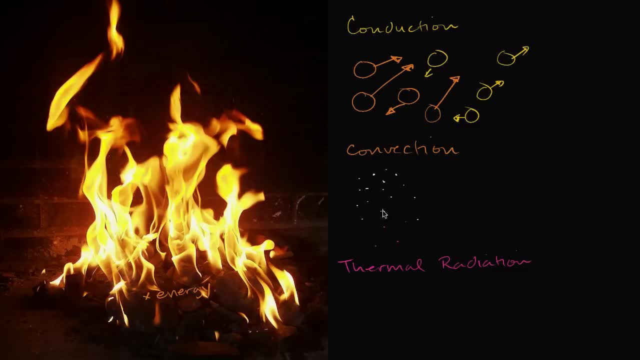 Because hot air, these particles have a much higher kinetic energy and so they're gonna bump into each other and they're gonna push each other much further away and get more separation from each other because of that high average kinetic energy, But because the hot area is less dense. 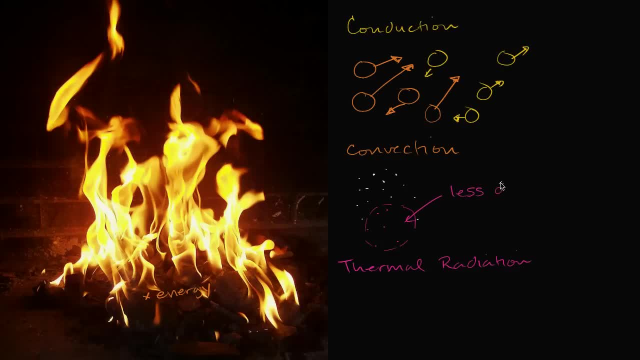 this area right over here is less dense- less dense than the white area. These might all be the same molecule. I just made them in different colors to show the less dense area and the more dense area. It is going to rise. it is going to rise. 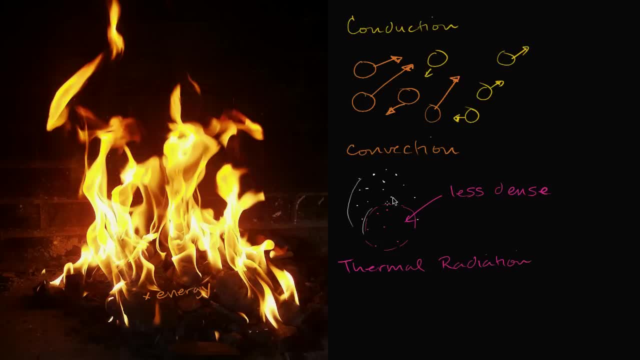 or you could even think of it as the more dense area, the more dense area is gonna fall around. it is going to fall around it, or try to go under it, because it is more dense, and then the less dense area is going to rise. 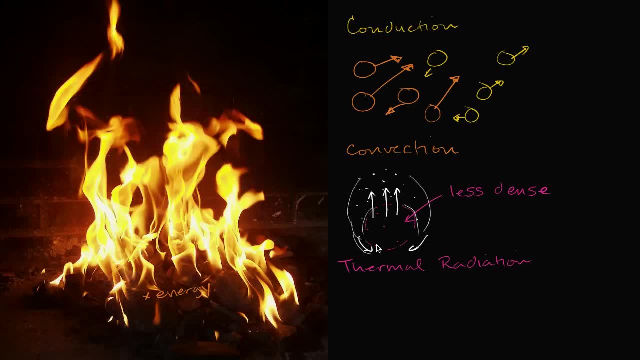 And by doing that you have the hotter molecules are moving upwards And then the cold molecules can go down to, maybe the source of heat. the source of heat, the source of energy right over here to get heated up more. So this right over here, so hot air rises. 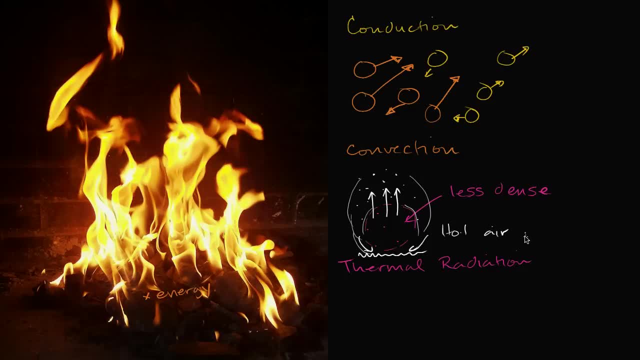 Let me write this: the hot, hot air rises And one way to think about it- it makes room for the cooled air to come down and then get heated up again. And that's what's going on in the fire here. You see the combustion reaction. 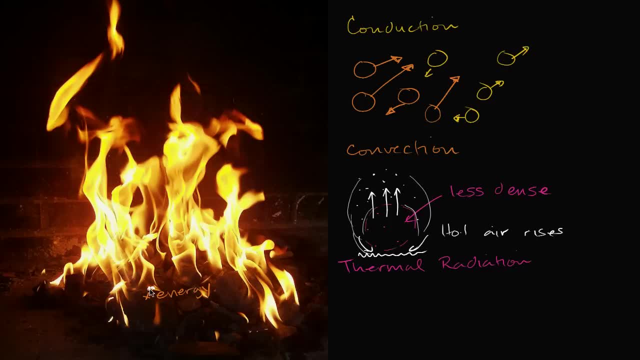 Combustion reaction occurs right over there. Let me do this in a different color. Combustion reaction is occurring in the fuel, that super hot air. it's going to rise And that's why it looks like these flames are kind of 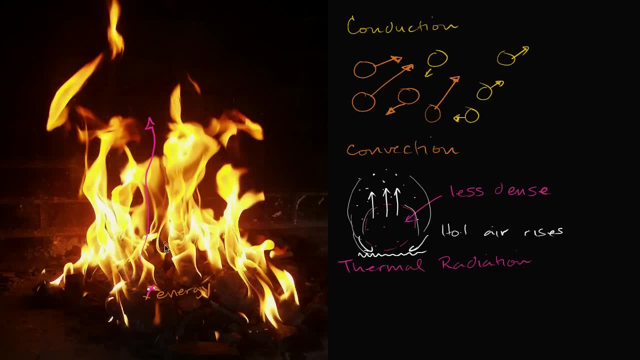 they're moving upwards, they're kind of flickering upwards And you'll also see- and actually we're gonna talk about this in thermal radiation is that they also change color as they move upwards. But this whole idea of fire moving upwards and the hot air, 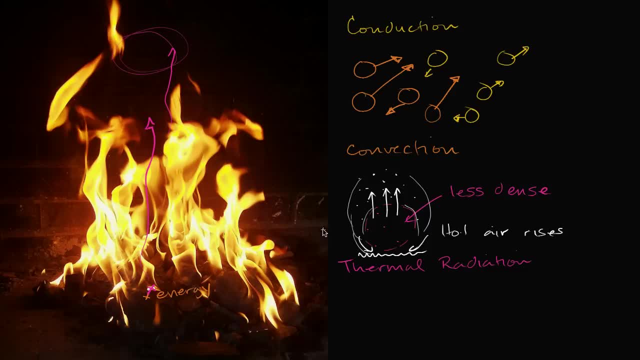 if you put your hand up here, it's gonna be much hotter than if you were to put your hand, than if you were to put your hand, say, right here, Even though in theory this is closer to the flame than up here, and that's because the hot air 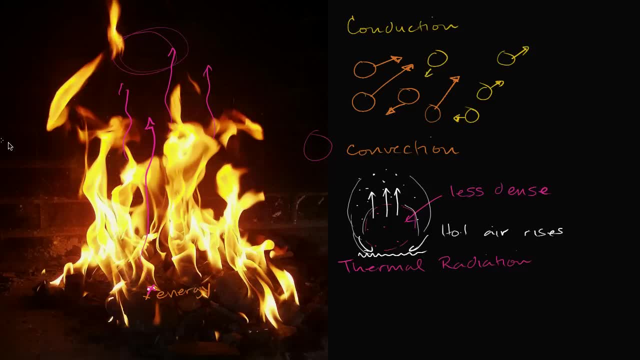 the hot air is rising and it's making room for cold air or cooler air. I guess I could say: come down here and be part and get heated up again, and then it would rise up again. And so this convection, this idea of the hot air rising, 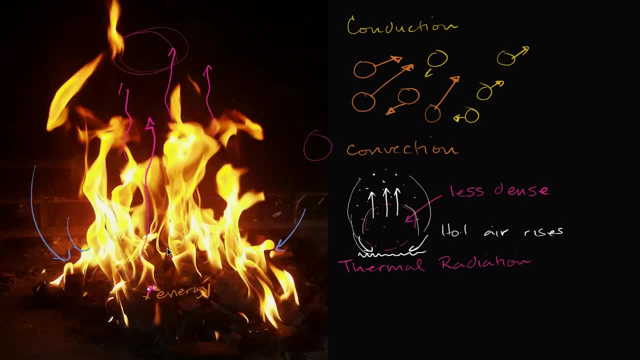 or the cold air falling. this is another form of heat transfer. Now, the last form that we're observing when we're looking at fire is thermal radiation, And this is all around the idea that if you have charged particles being accelerated, they're going to release. 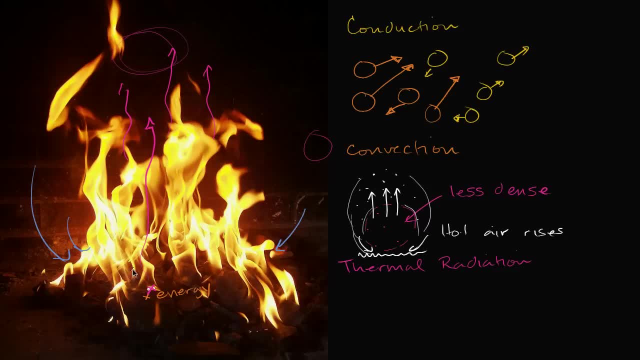 electromagnetic radiation. And so you might say, wait, wait. charged particles, where are those being accelerated here? Well, we have these molecules that are constantly being accelerated as they bump into each other. One's gonna transfer kinetic energy from, let's say, this, one bumps into that. 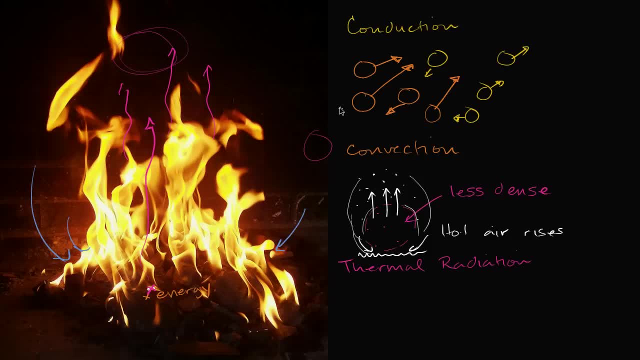 it's going to accelerate that in a different direction, And even this one might go in another direction, and acceleration is a change in velocity, So it could be the magnitude of velocity or your direction of velocity. So, as they're colliding, you have all of these. 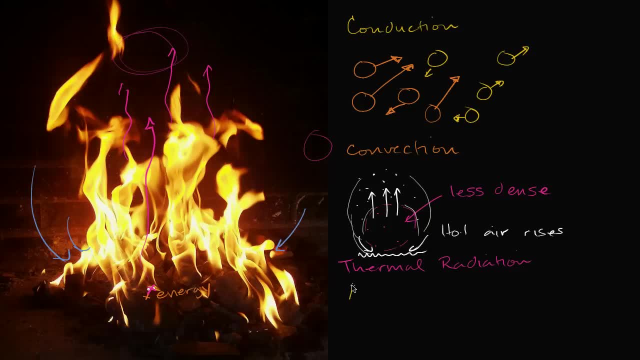 acceleration of charged particles. so let me write this down: You have acceleration of charged particles and then that releases electromagnetic radiation. I know what you're thinking. wait, wait, hold on a second Sal. okay, I can buy that. we have molecules that are being accelerated. 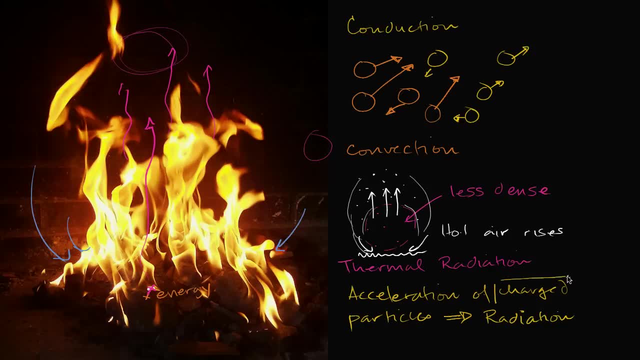 but where is this? where is this charged? where are you getting this charged particles business? Well, we have to remember these molecules are made up of atoms and atoms are made up of charged particles. they're made up of protons and electrons. 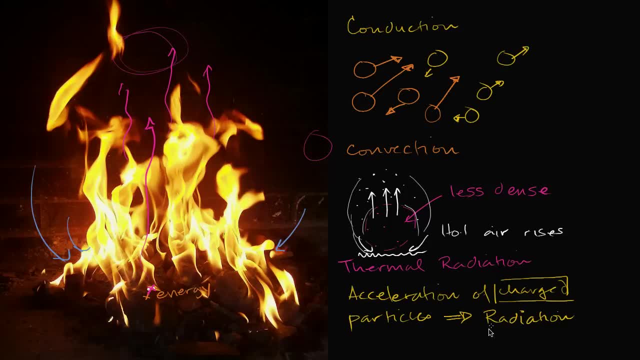 And so as you accelerate these, and the more that you accelerate these, the more radiation you are going to release. And you might say, wait, wait. okay, you said I'm observing that in fire. where am I observing radiation? Well, just the very fact that you can see the fire. 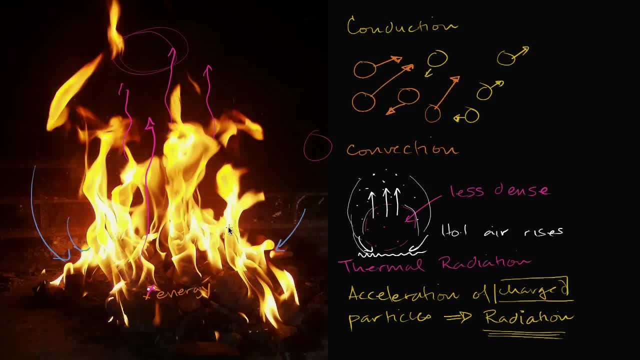 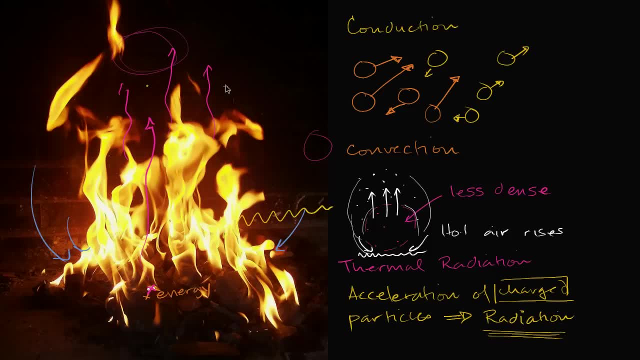 Even the particles up here. so even the particles up here that are still quite hot. they are also emitting electromagnetic radiation because they're all bumping into each other and their electrons and their protons are all getting accelerated in different ways, They're also releasing electromagnetic radiation. 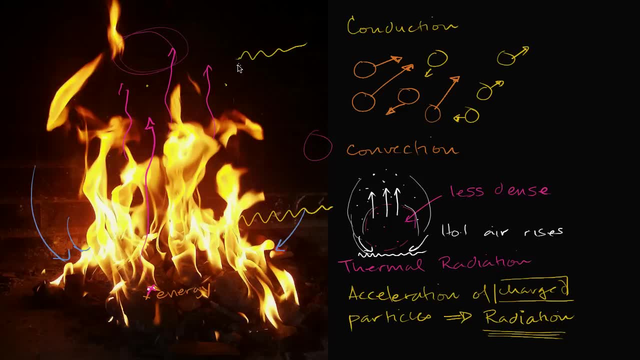 but it is at a slower wavelength than your eye is capable of perceiving as light. If you had an infrared camera, you would see the flames being much larger. You would see them go all the way up here, And if you were to look at the flame closely, 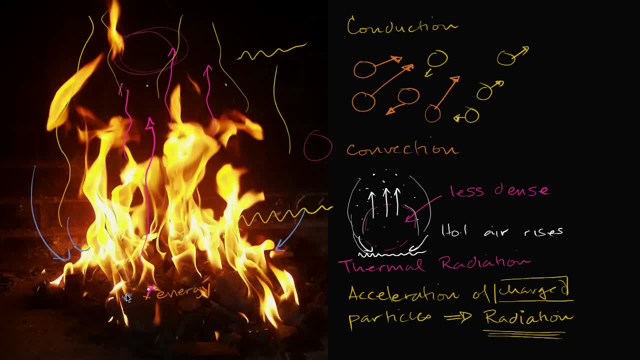 you would see down here right where the combustion reaction is happening. the flame looks blue And that's because the blue light is higher energy light and that's because the particles are being accelerated more down here. and then it goes from blue to kind of white, to a yellow, to a red. 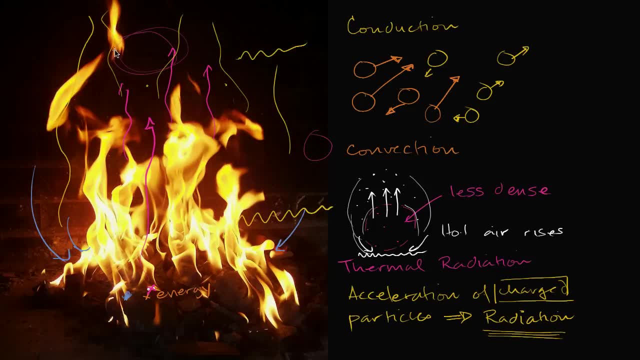 or to an orange, to a red and then to your regular eyes, it disappears. but everything, everything that has some temperature, is releasing electromagnetic radiation And you're like, okay, well, that's all fine, I can see it, but how is that a form of energy transfer? 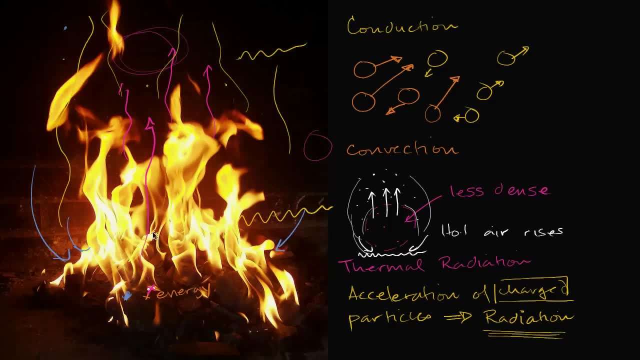 Well, if you've ever sat next to a flame, you will feel the heat. In fact, even if the air between you and the flame is cold, you would still feel like you're getting warm. So if this is a flame right over here, so that is fire. 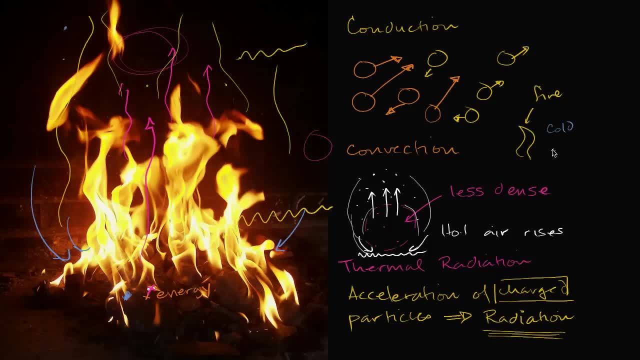 and let's say you have cold air, cold air. let's say you're at a campfire right over here. maybe it's 30, this air right over here is 30 degrees, if you are, if you are standing right over here. 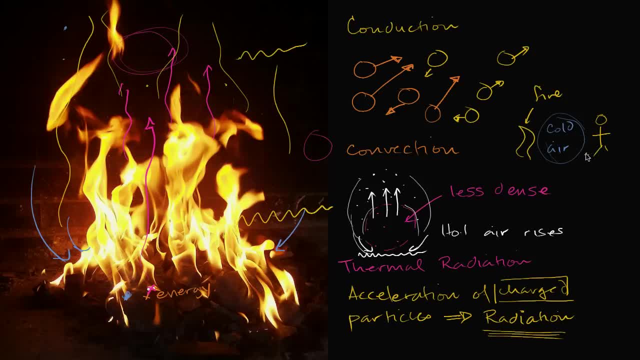 you would still feel heat, you would still feel like you're getting warmed up, and that's because that electromagnetic radiation is being emitted from the air- particles that we perceive as fire- and then that can actually excite particles on your skin and it'll transfer energy to your skin. 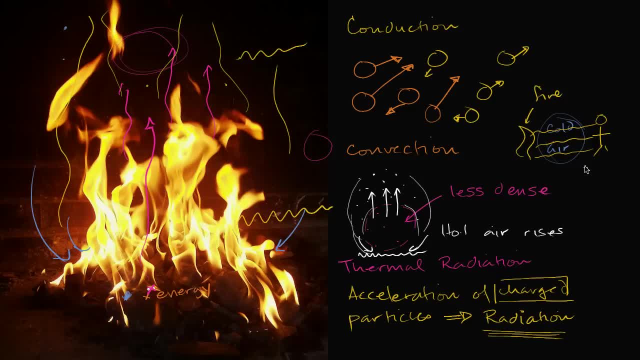 And so you feel like you are actually getting warmed up. I remember once- this is kind of a strange story, but I was on the highway and there was a car on fire and I was. literally we drove to the far lane because it was on fire. we're three lanes away from it. 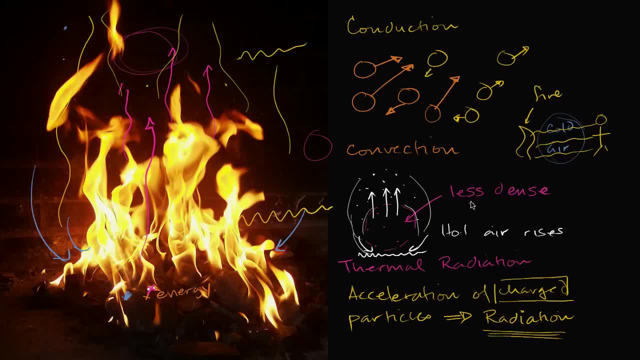 and it kind of exploded. I don't think anyone was in it. hopefully no one was in it- but I remember right when it exploded, it was an intense, immediate heat that we felt through the window of the car and that was electromagnetic radiation. 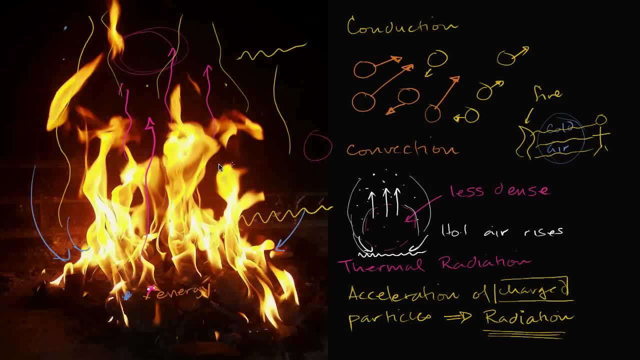 That was thermal radiation, Radiation being released by these accelerated particles in the air around that explosion, which we perceived as an explosion or fire, but then it was warming up particles on my skin.